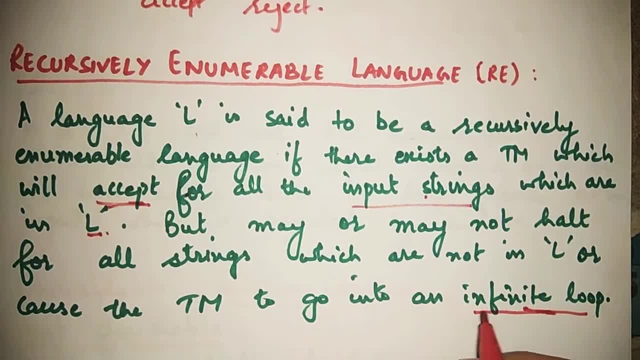 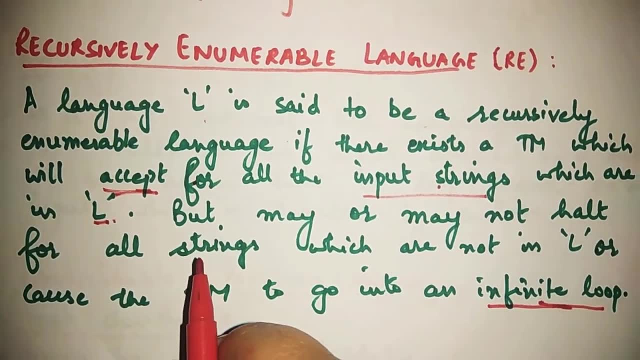 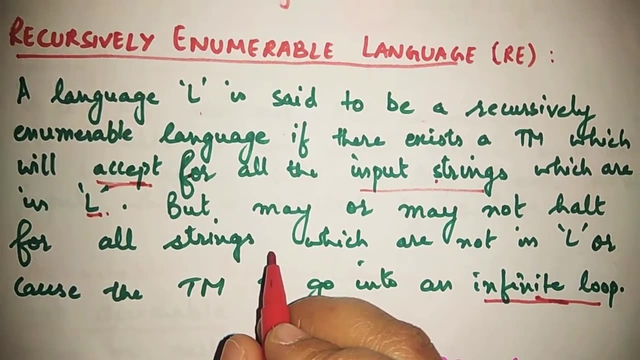 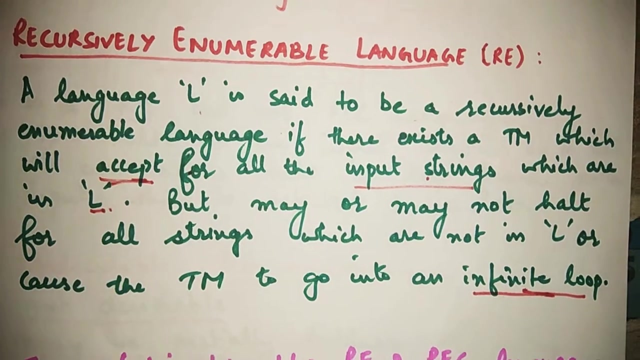 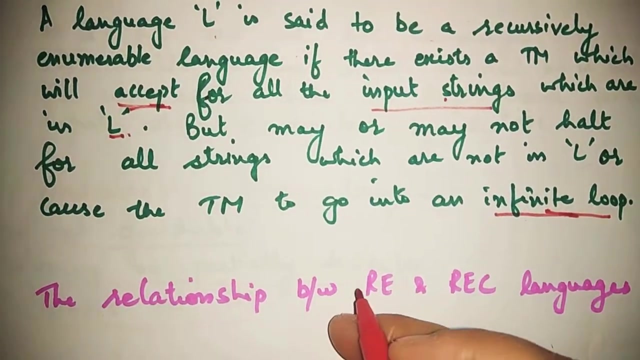 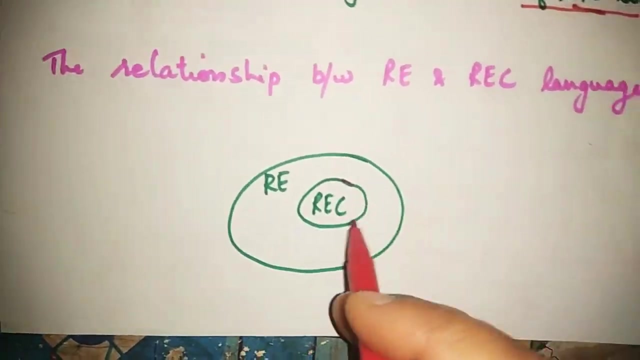 an infinite loop. so what does it mean in this? sometimes the Turing machine will hold and sometimes it may not hold. so in that case it will not guarantee that Turing machine will always accept or reject. so what we have discussed, so in recursively language, enumerable language or recursive language. so what is the difference between these two? we can say: 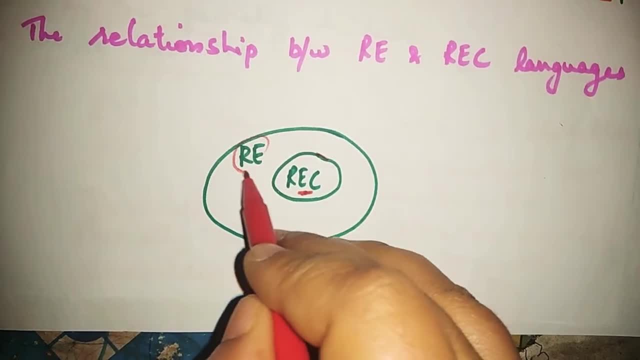 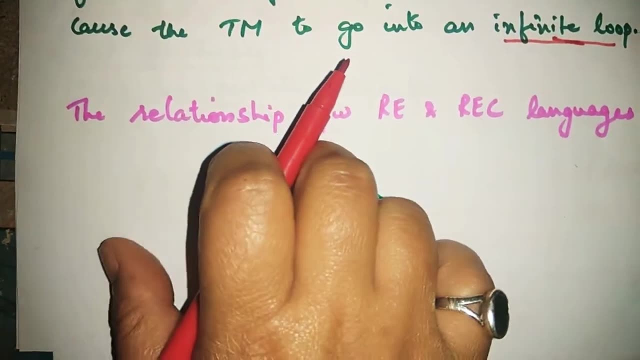 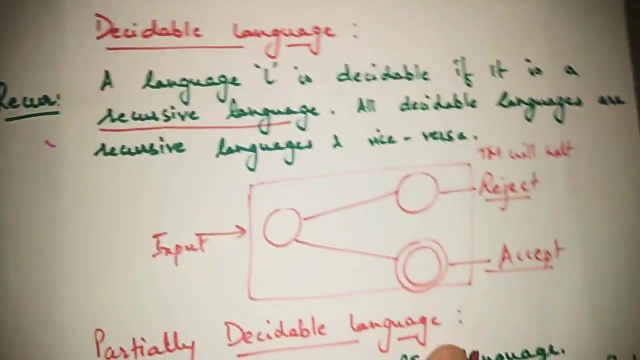 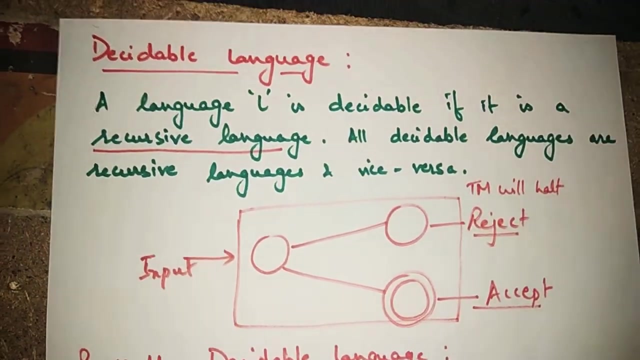 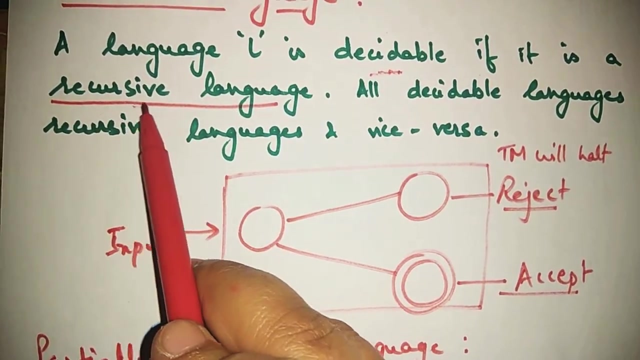 that recursive language is a subset of recursive enumerable language. so by considering these two language, we can now study what is a decidable language and undecidable language, or partial decidable language. so a well, What is Decidable Language? Language L is Decidable if it is a recursive language, and we have already discussed that. 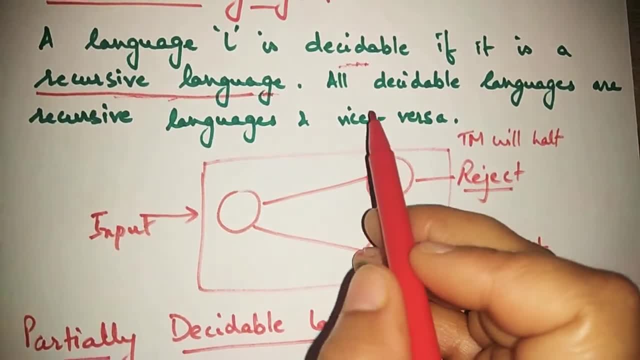 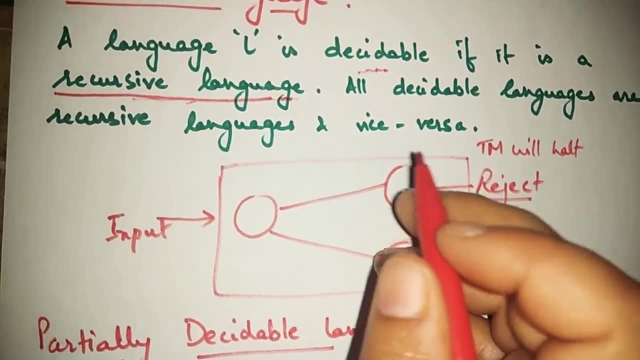 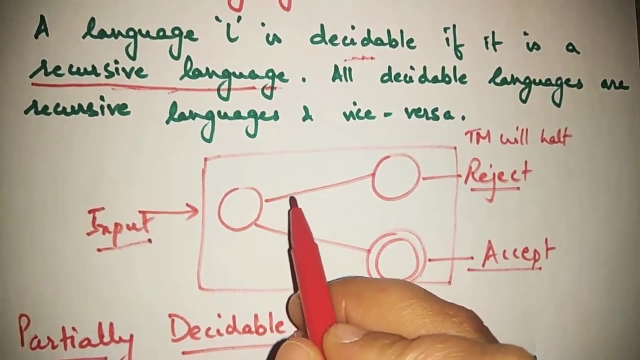 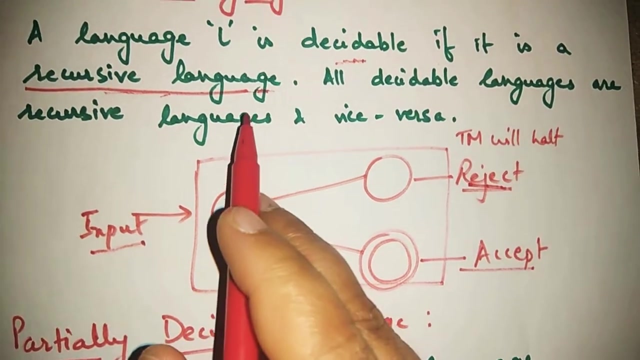 what is recursive language. So in this case the Turing machine will always halt or give or reject or accept the string. So when we pass a string then it will always halt. That means it will reject when the string doesn't belong to the language L and accept. 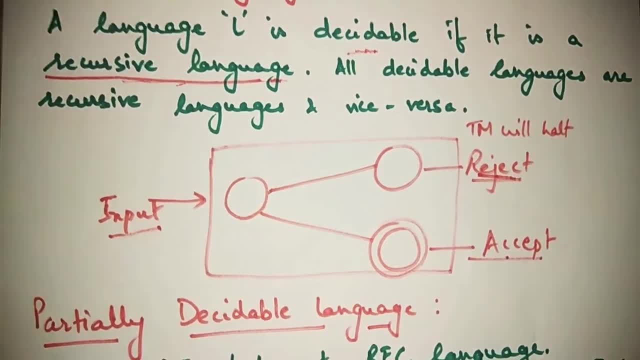 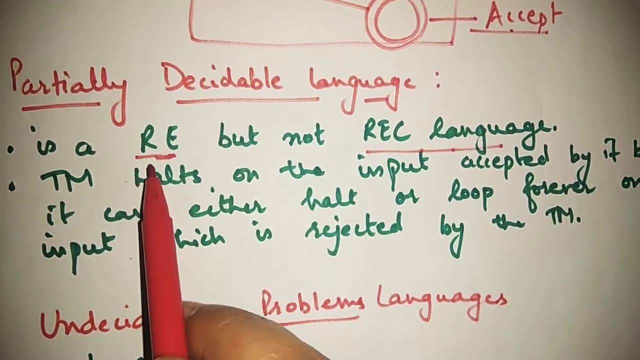 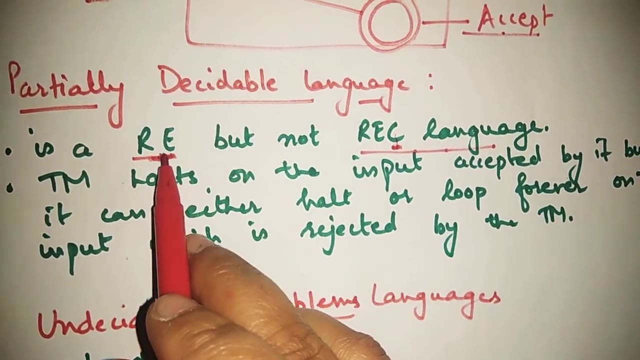 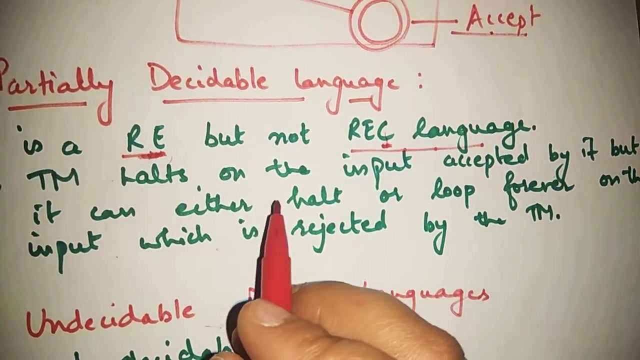 when the string belongs to language L And another language is Partially Decidable Language, It is a recursive enumerable language but not recursive language. So in that case it may halt or may not halt or sometimes go into the loop forever. We have already discussed the meaning of recursive enumerable language. 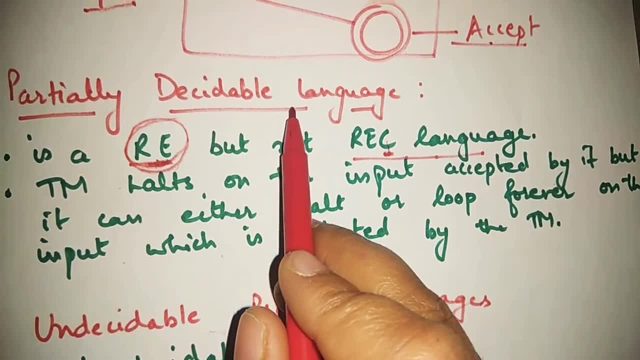 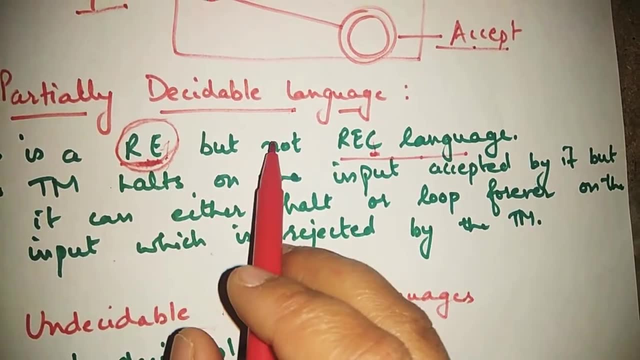 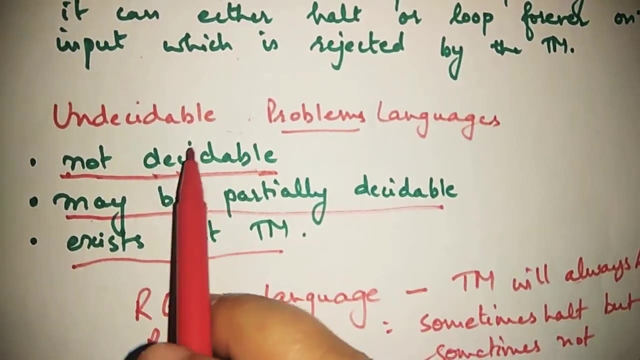 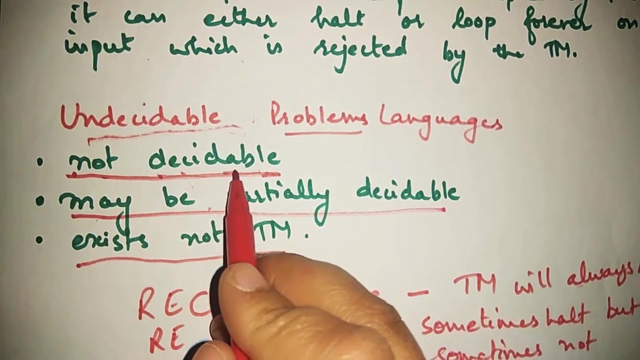 So in this case it may accept when the string belongs to the language L, or in other cases it may not halt or go into the loop. So another. We will discuss Undecidable Problems or Language. So what does it mean? It means that it is not decidable.